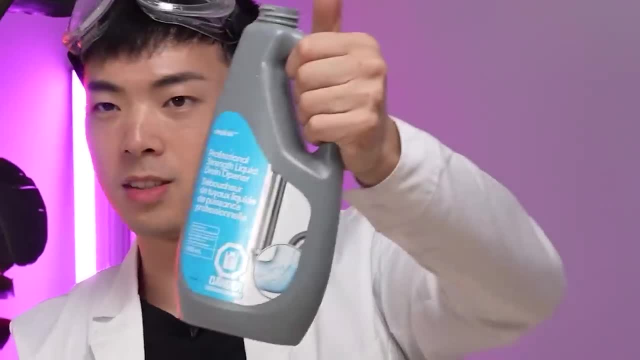 gonna put a giant balsa in here, and we're gonna put a giant balsa in here and we're gonna put a two aluminum can experiments. For the first one, we just need some drain cleaner Stuff. you can buy at the hardware store. 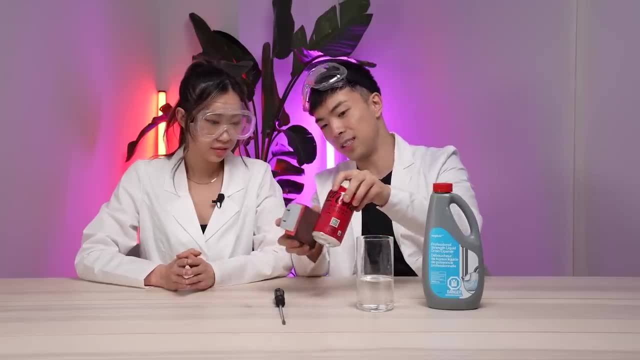 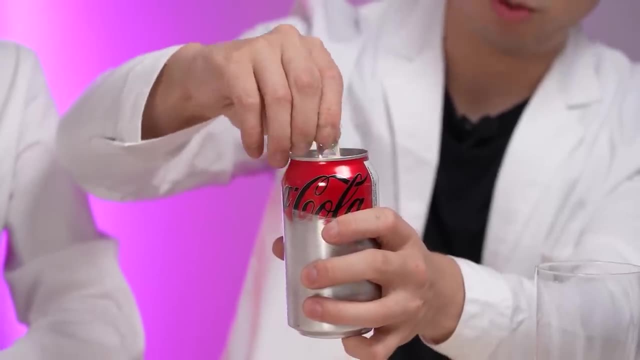 I'm gonna fill this up Now as my assistant. I need you to sand this Coke, can? That's pretty good. Now we've sanded off all the labels. Ooh, we're gonna put this in Instantly dissolving. that's crazy. 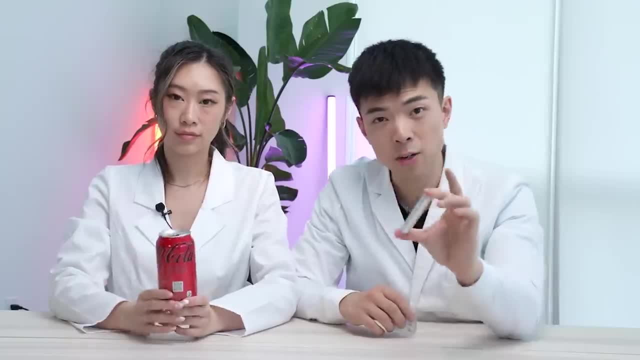 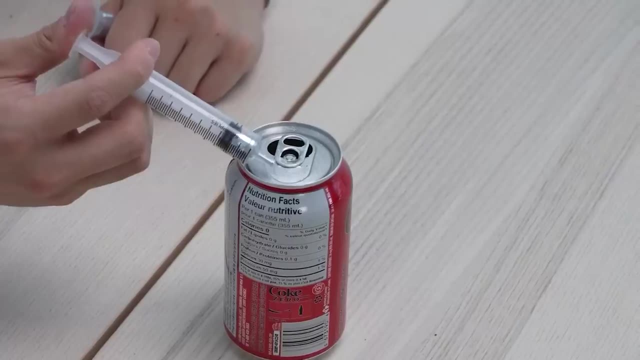 Up next is aluminum can versus gallium. So the special thing about gallium is the fact that when it comes in contact with any aluminum surface, it will melt the aluminum. We can put the gallium on top. Why don't you spread it around? 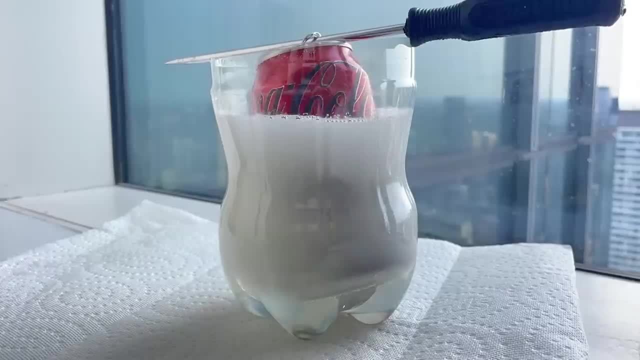 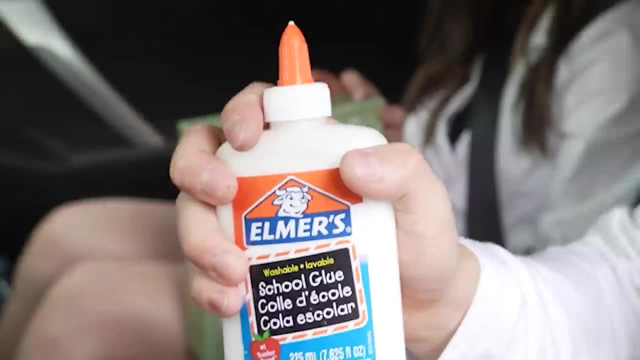 Safety touch. We'll need some time for the melting process to happen, so we'll check back on both aluminum can experiments later in the video. This next experiment needs to be done in the car. We'll just start with some Elmer's glue. 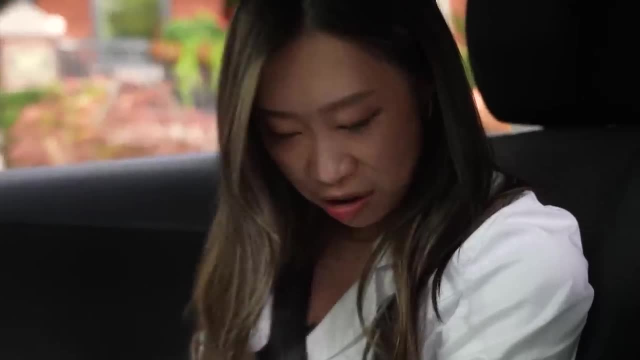 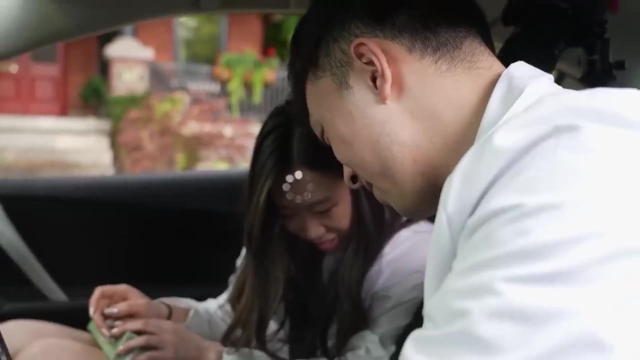 You're pouring glue in the car Halfway. are you sure you're gonna be able to get that out? You gotta trust science. Pour this into the cup, shake it up. Let's hope this works. What if it goes into the engine? 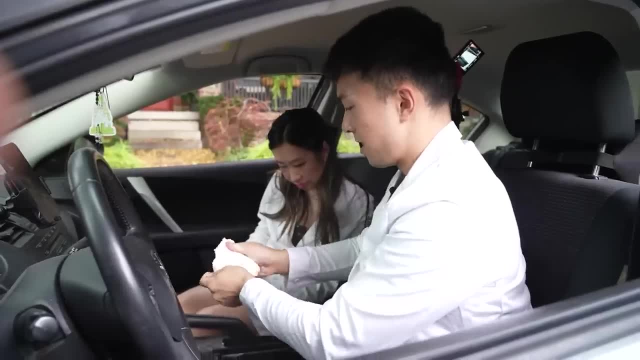 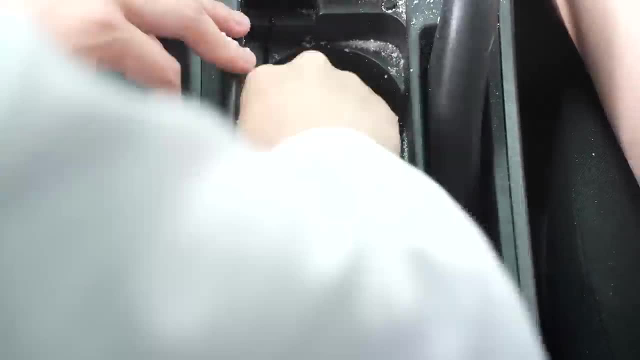 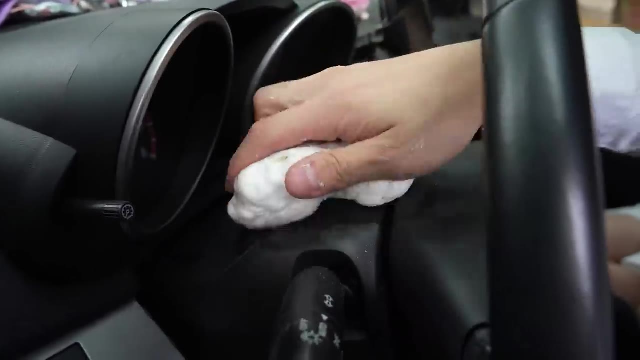 Into the engine. All right, we have our beautiful slime. Now this should clean our car: Clean the cup holder, Clean up some dust here. Clean up some dust Now. let's clean the steering wheel. Look at that, it's sucking everything up. 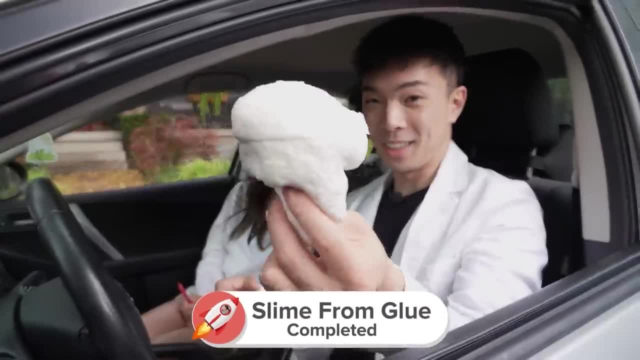 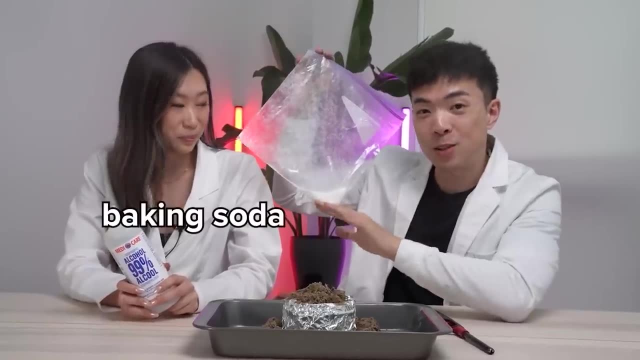 That's so gross. Now we have a brand new car completely cleaned with glue. This next experiment is the carbon sugar snake. This is our snake, right here. It's just a mix of baking soda and sugar. What I need you to do is pour the rubbing alcohol. 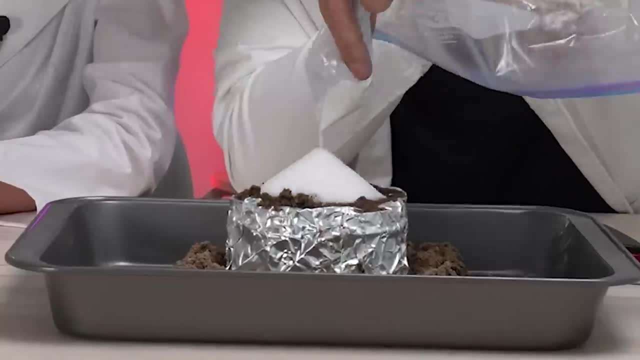 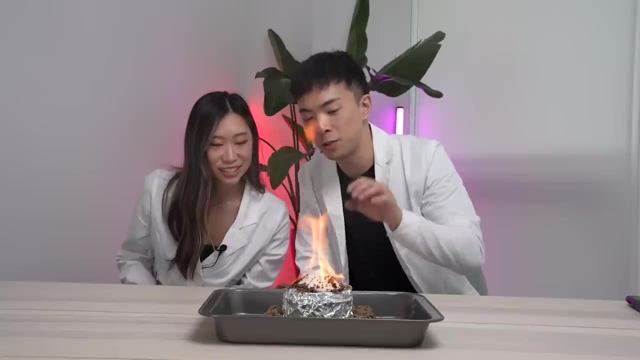 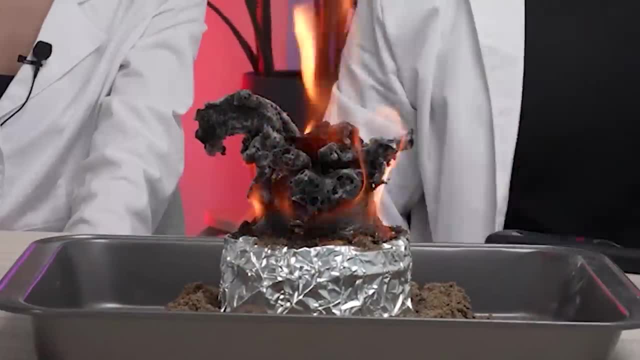 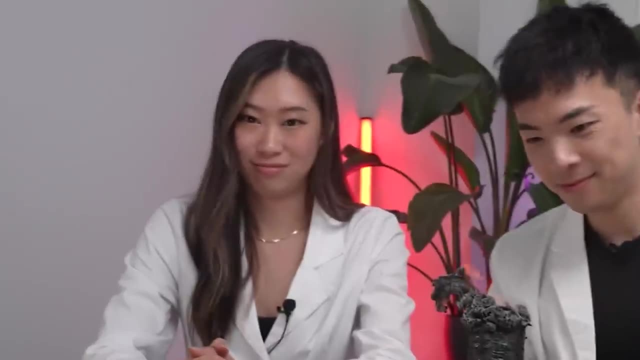 As the mixture burns, the carbon dioxide gas is getting trapped inside, which is making the sugar come alive. What are you gonna name your monster? Hapu Big Willy? I'm sorry my man, Cool thing about this: you can actually touch it after. 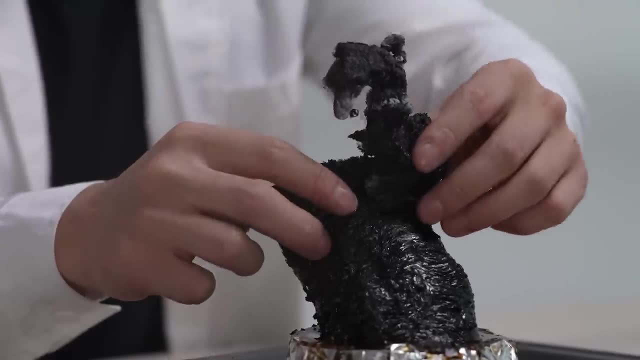 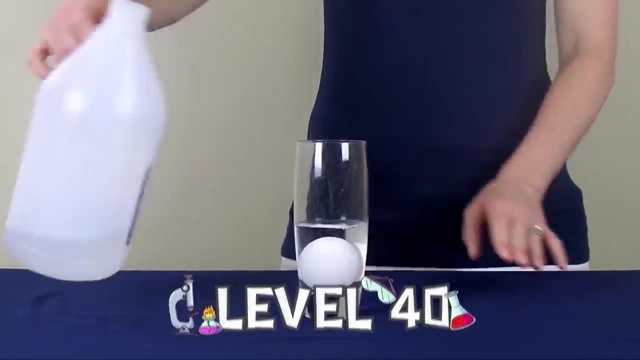 It feels like a croissant. Yeah, You can like, peel it open, spread it open. We basically made bread. All right, onto the next experiment. This next experiment only involves a simple egg. This is what happens when you drop an egg, normally. 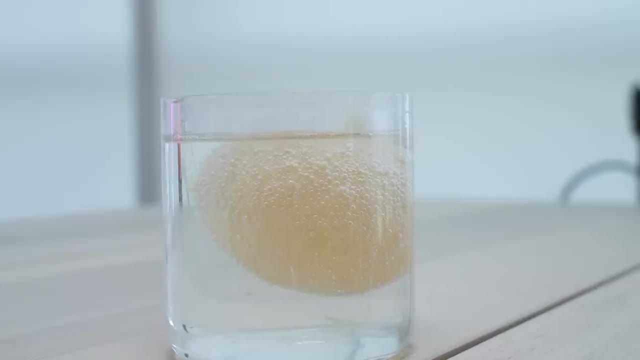 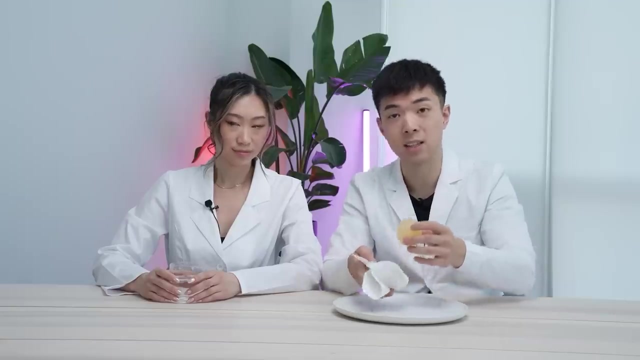 It breaks, as expected, But when you put an egg and soak it in vinegar for two days, it breaks. In this case, this is what happens. Our egg is now see-through, And what happened here is the acid in the vinegar has actually broken down the hard parts of the egg shell. 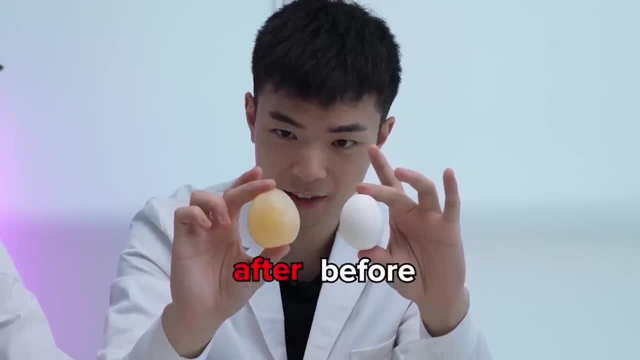 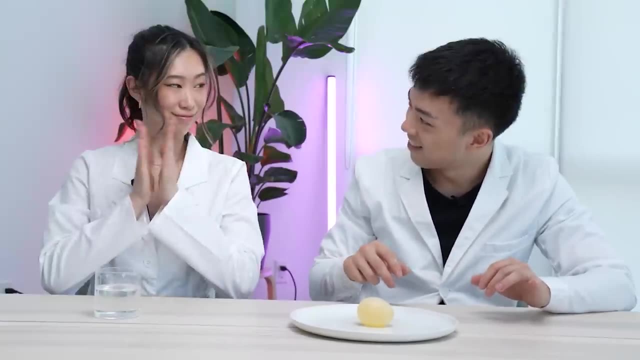 which became these bubbles. This is a before and this is an after. Now, what's left intact is a membrane inside, so the egg is actually bouncing. Look at this. That's so cool. Let's make a bet. Loser has to eat this. 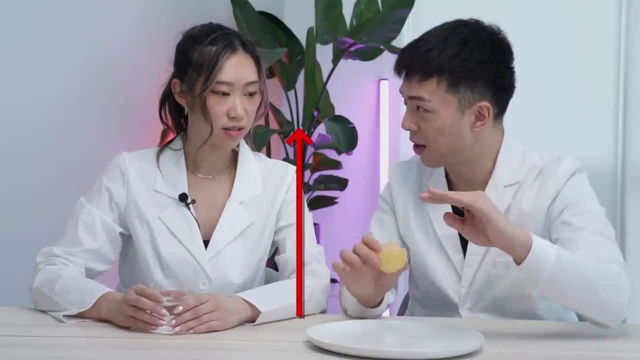 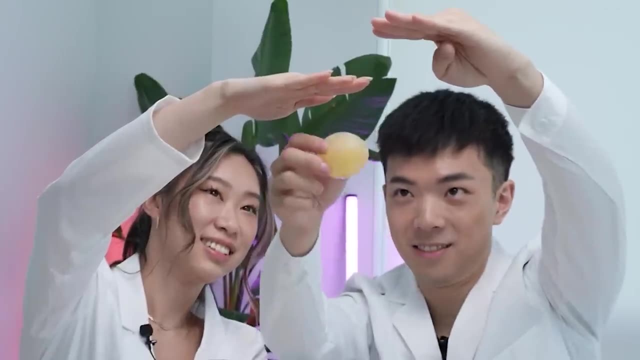 Make a bet on how high you think this egg can bounce without breaking. I'm gonna say two, Two. I'm gonna say here. You're gonna say higher than me, Okay. then I'm gonna say here: Okay, ready, We'll go here first. 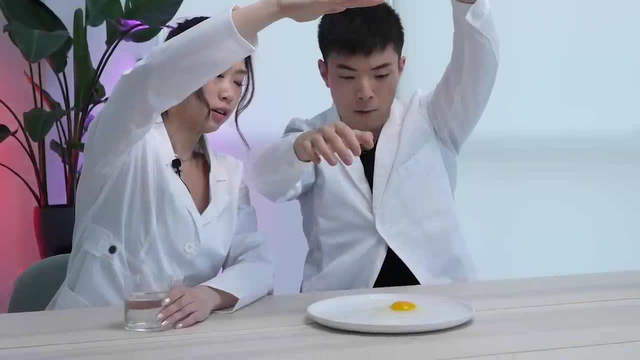 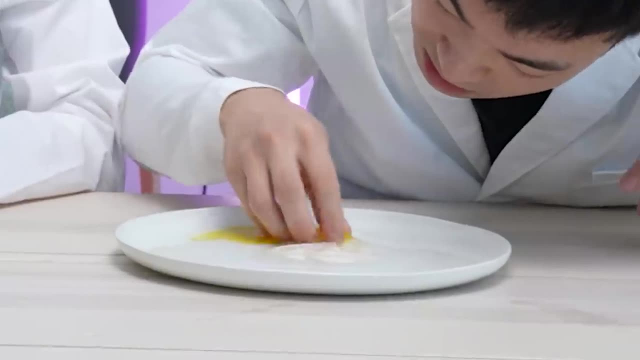 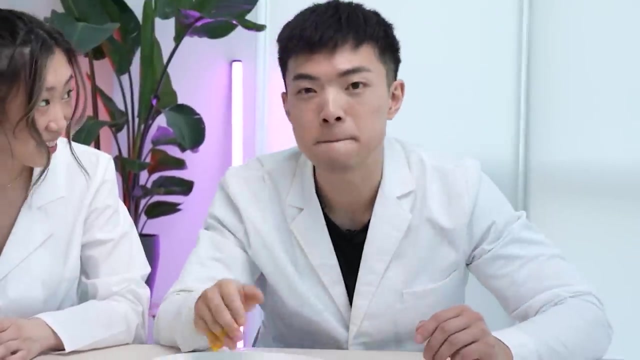 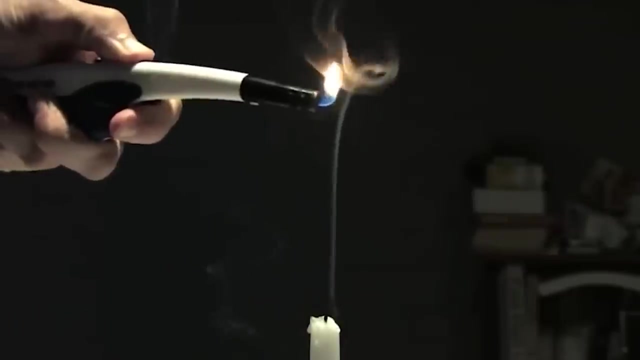 You're eating the egg. I'm closer. Oh, that's disgusting. That is actually disgusting. You're eating the egg. Honestly, it just tastes like pickle. Pretty cool science experiment, Very easy to do. Next, This is a normal lighter, but we're gonna turn it. 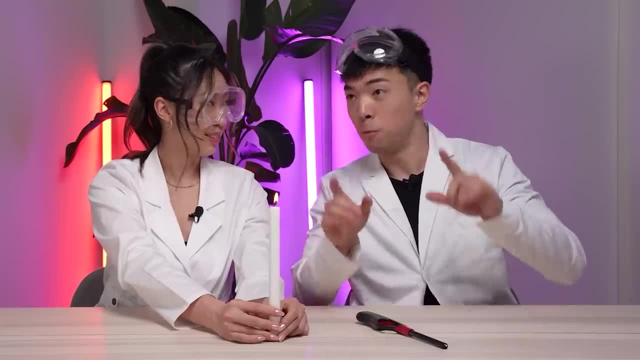 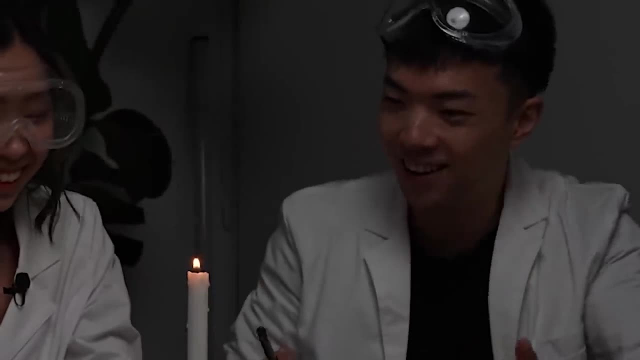 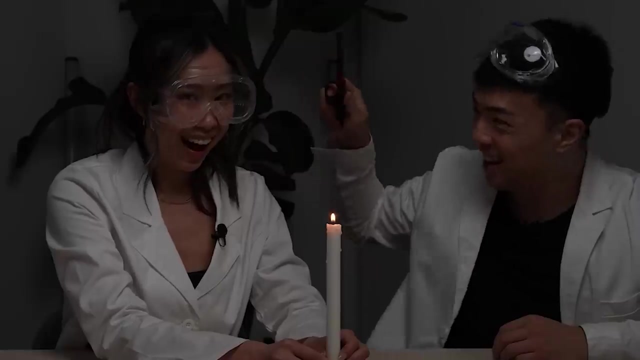 into a magic lighter. All right, What does that mean? We need the lights off. So what I'm gonna need you to do is just blow Harder, Blow harder. Did you see that? Yeah, that was really cool. So when the flame blows out, there's actually. 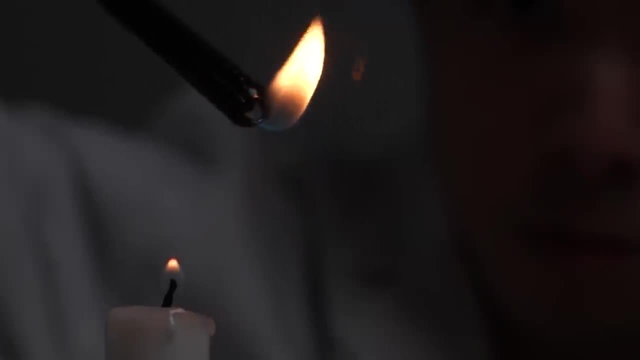 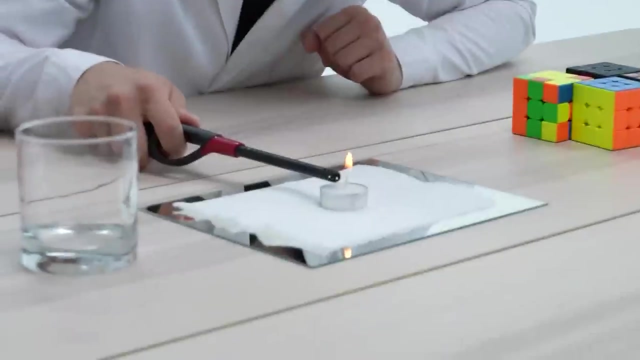 leftover wax in the smoke. That's why, when you add heat, it will relight on fire. This next experiment is called fire suction, So I'm gonna need your help later. First, we're just gonna light this candle. Pour a little bit of water around the 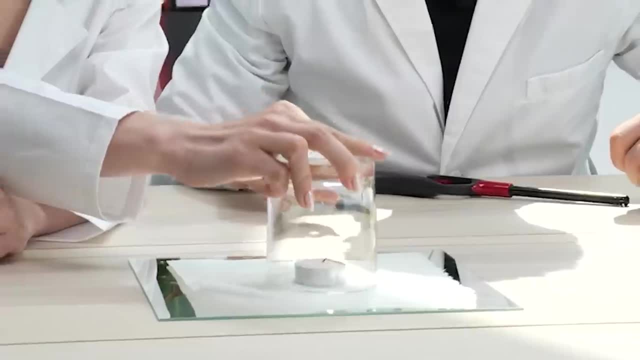 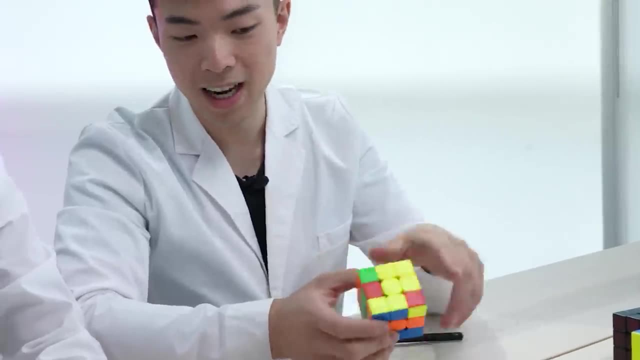 I said a little bit, Place this on top, Place a glass over it, which is gonna create a suction once the fire dies out. And while we wait for the fire to die out, I'm gonna solve this Rubik's cube so we can test the strength of this suction. 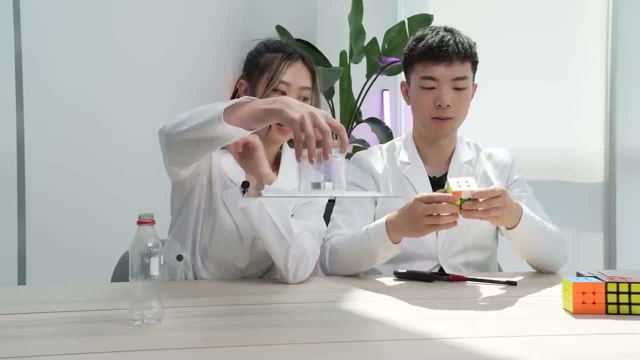 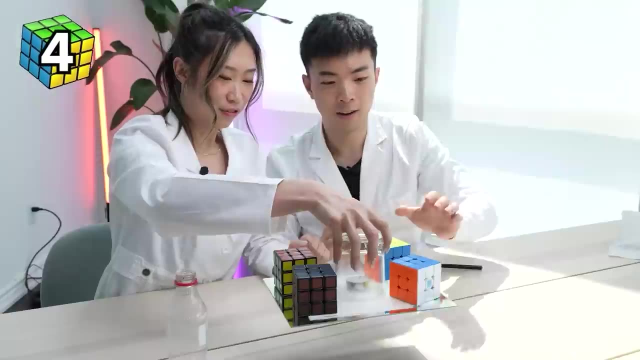 Ooh, Yeah, it's working Nice, Place a Rubik's cube on top. Yeah, Okay, One, two, three, Last one, All right out, All right, there we go Four. What else can we place on top? 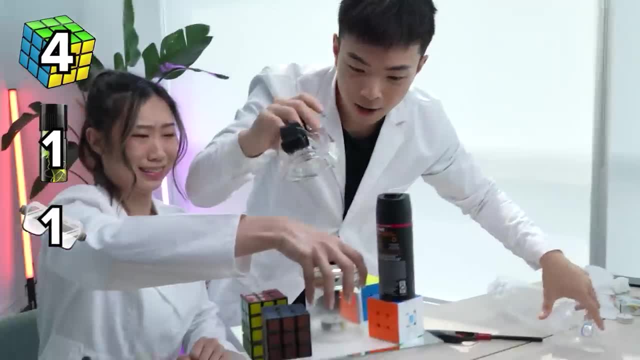 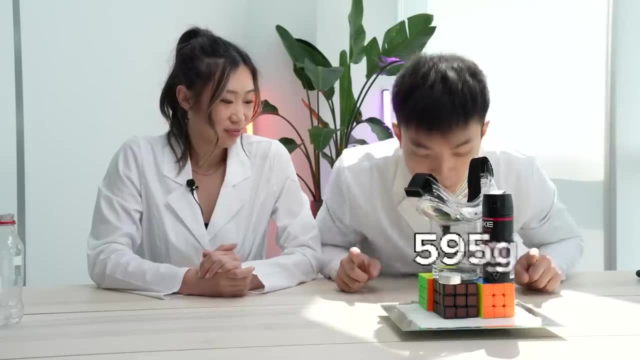 Can we place this axe can on top? Can we place this goggle on top? Can we place- oh okay, Now we can weigh out everything on top, and that's a total of 1,161 grams. The power of this tiny little candle. 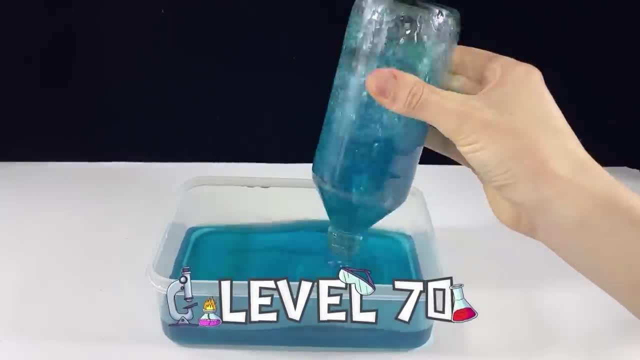 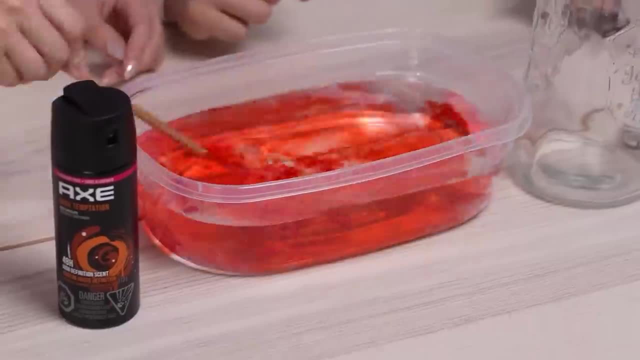 Next experiment. This next experiment is called water suction. Should I be concerned? Just a little? You're gonna put some food coloring in this water, just so it's visible. Swirl it around And now we're gonna make me 10 times more attractive. 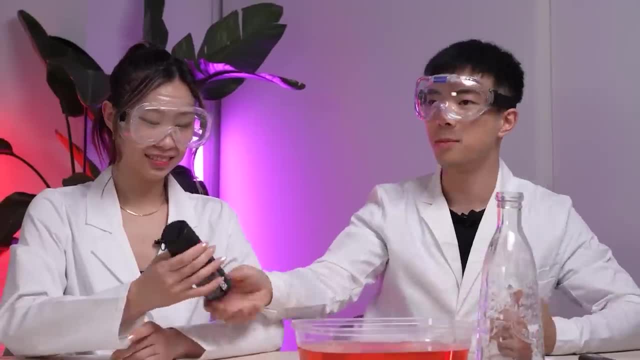 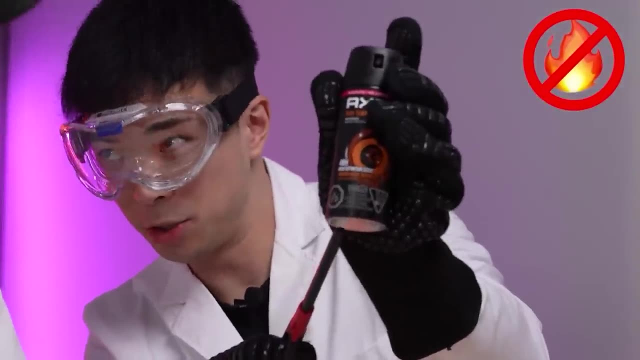 This is Axe Body Spray. Every high school man's dream Spray me. How does it smell? No, On the can of Axe Body Spray it has a fire emoji. Whoa, That's cool, Kinda like a flamethrower. 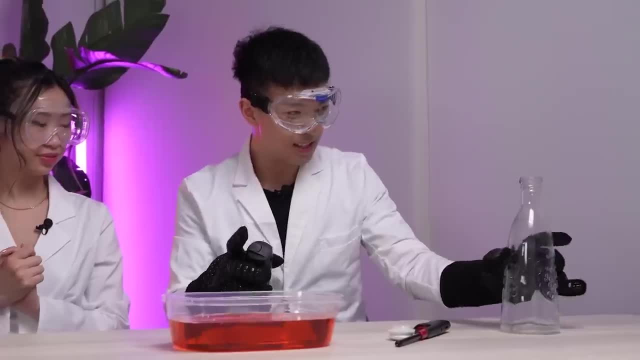 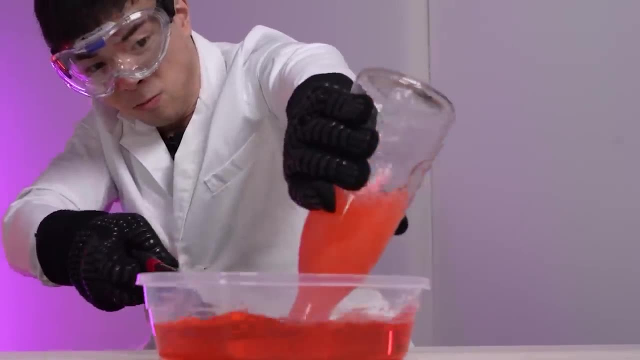 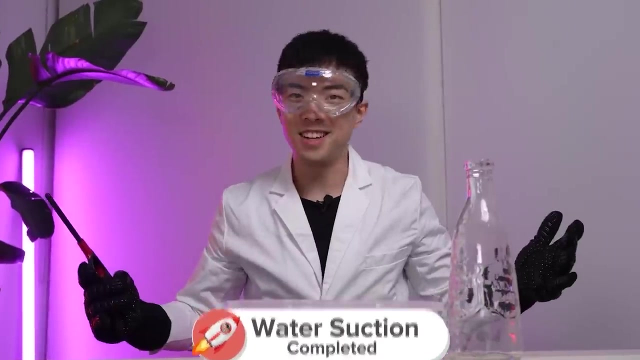 But that's not our trick. Our trick is: we're gonna use this inside of the bottle, Just a little bit. All this water will instantly go into the bottle once I light this. Whoa, And that's water suction. Is fire suction cooler or water suction? 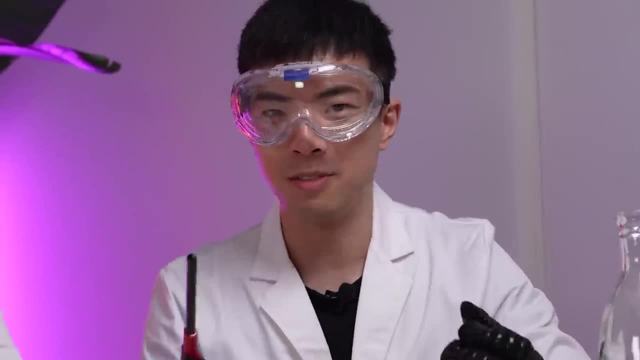 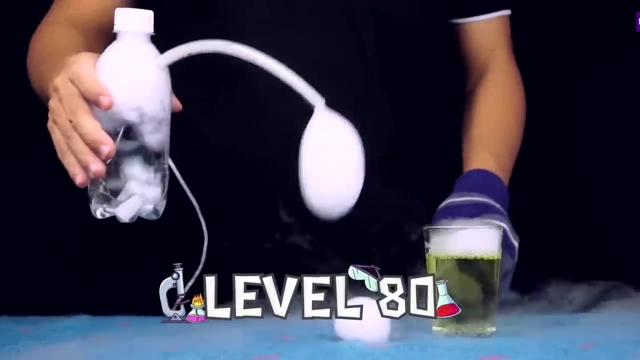 Water suction. When we're sucking, it needs to be a little wet for it to be fun, right Yeah, especially when it's red. Next experiment: So now we're gonna make a dry ice bubble maker. all right, When we put dry ice in water, we're gonna make a bubble maker. 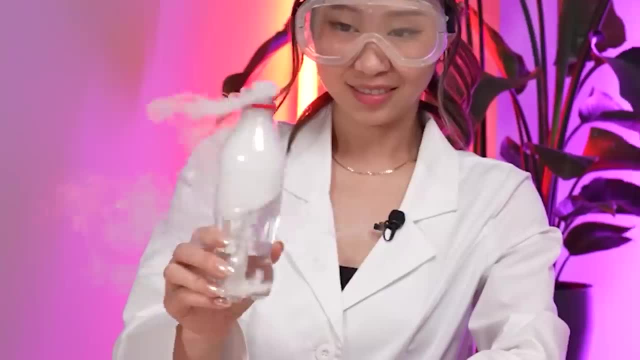 When we put dry ice in water, we're gonna make a bubble maker. When we put dry ice in water, we're gonna make a bubble maker Starts a reaction. Look at that, That looks pretty cool. We're gonna now screw on the cast. 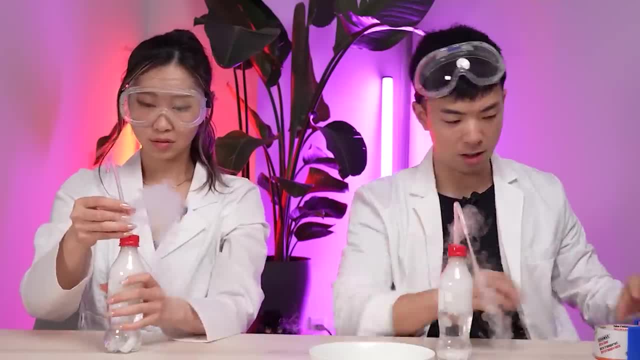 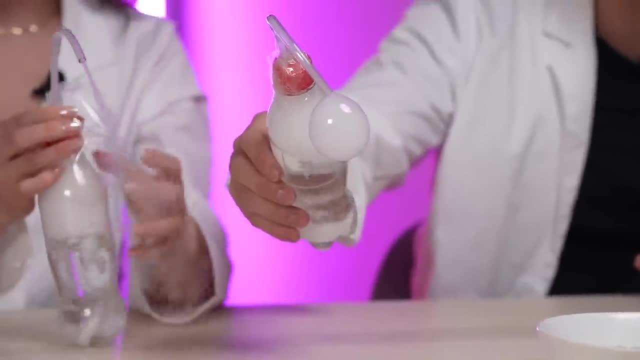 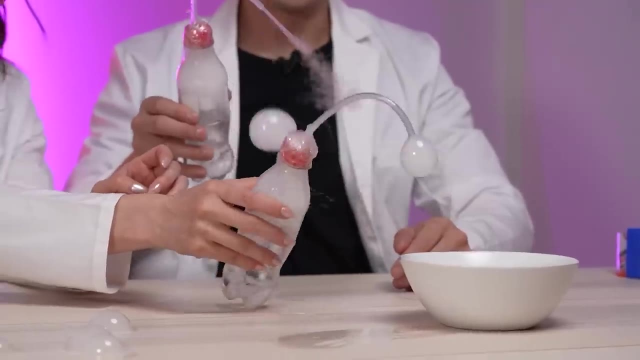 And then stick the tube in Not too far, though just a little bit, And we'll just tape it. Look at that dry ice bubble- Woo, It bounces. We're dipping the tube into a dish soap solution. The dry ice smoke gets trapped in the dish soap. 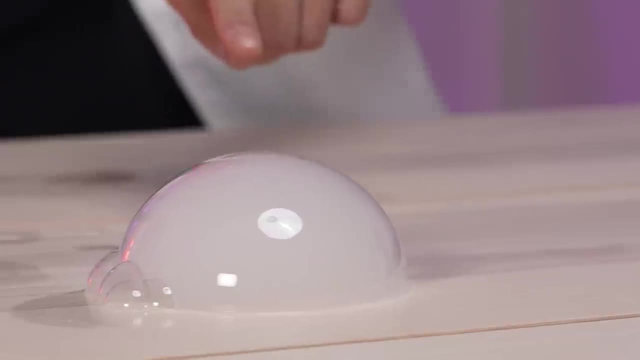 which starts to form a bubble, And our goal is to make the biggest bubble in the world. And our goal is to make the biggest bubble in the world. And our goal is to make the biggest bubble in the world. We can't. That's the process. 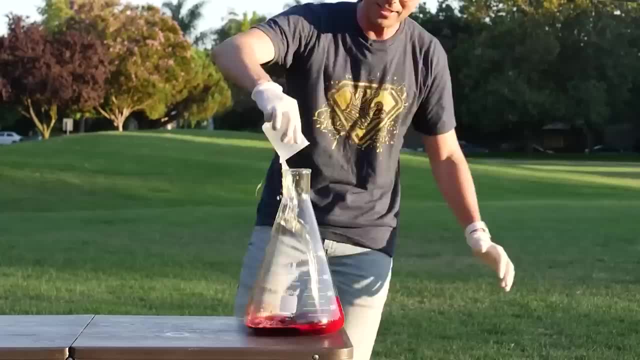 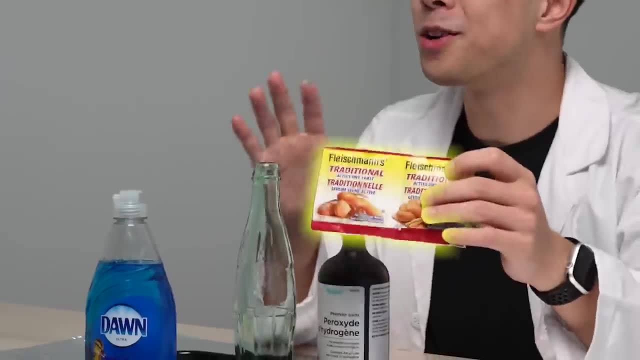 Look how big this is. Look how big this is. Oh, Next we have a chemistry experiment. I'm gonna show you how to make elephant toothpaste with just grocery store ingredients. All you need is some yeast, hydrogen peroxide, which is for wounds, an empty bottle dish soap. 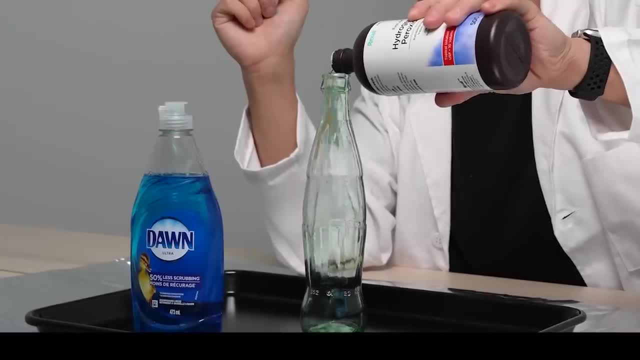 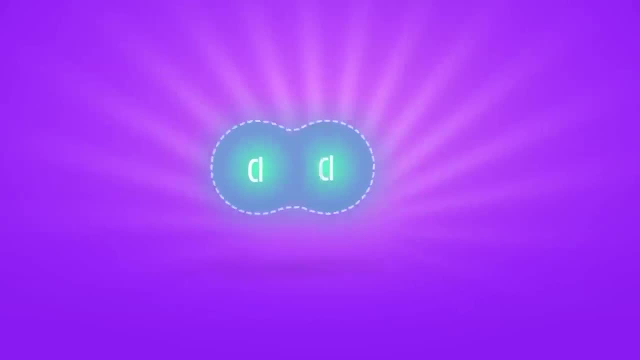 and food coloring of your choice. So first we just pour the hydrogen peroxide in here. Talking about chemistry, coffee season is actually coming up, So if you're still single, now is the time to form a bond: No more crying yourself to sleep at night. 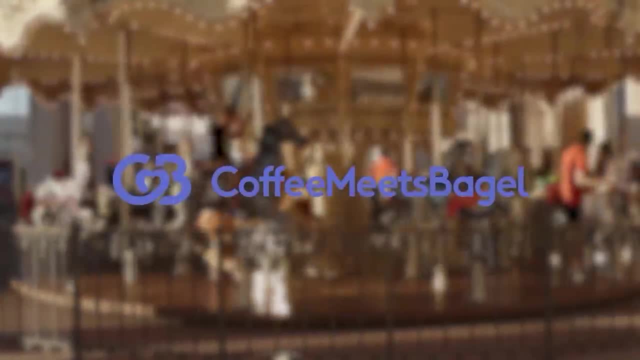 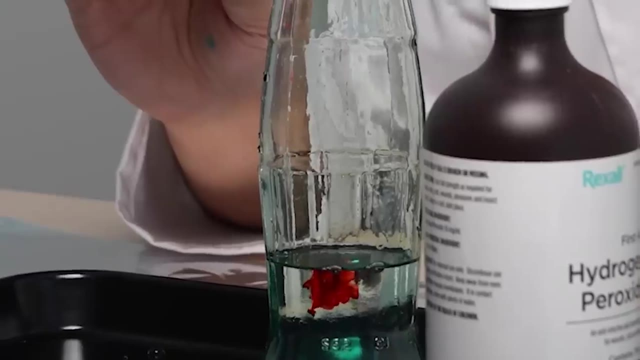 or bingeing shows alone. Our sponsor, Coffee Meets Bagel, is here to help. Let's add a little bit of dish soap And I'm gonna add a dash of red food coloring to signify love. So Coffee Meets Bagel is the last dating app. 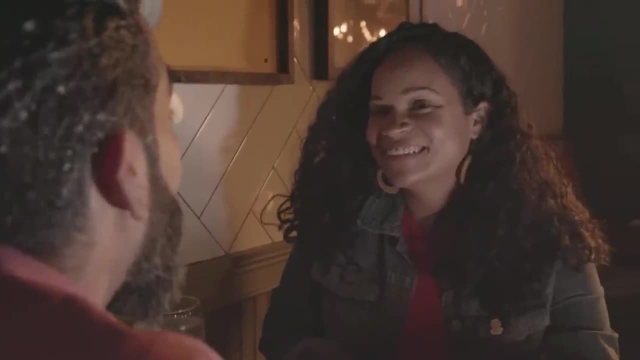 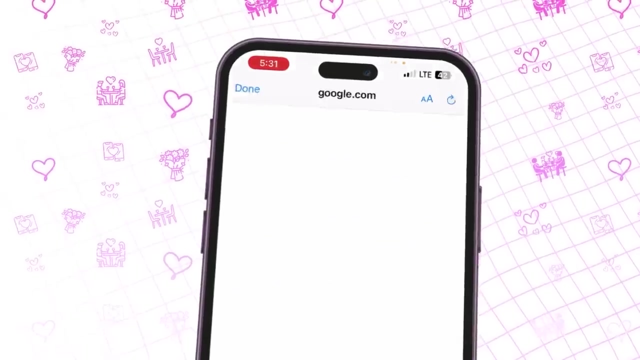 you'll ever need. It's made for those only looking for serious relationships. If you download the app and you say you're looking for something casual, they'll actually redirect you to competitor dating apps. I'm a very career-focused person and I'm sure a lot of you are just like me. 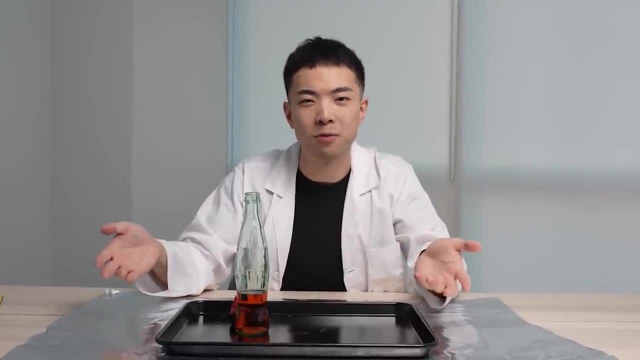 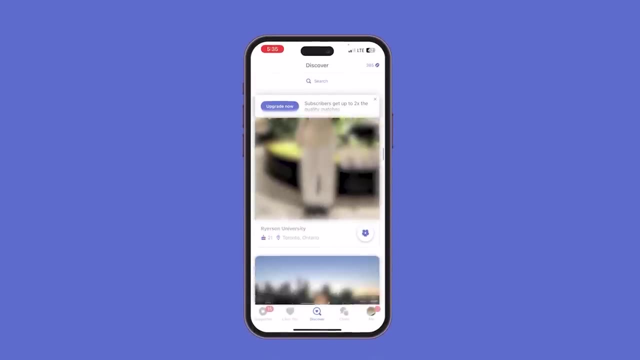 So swiping through profiles might seem like a waste of time for you. That's why I love Coffee Meets Bagel's matching feature. Instead of endlessly swiping, you get suggested new matches based on your dating preferences. For example, you can say you like girls. 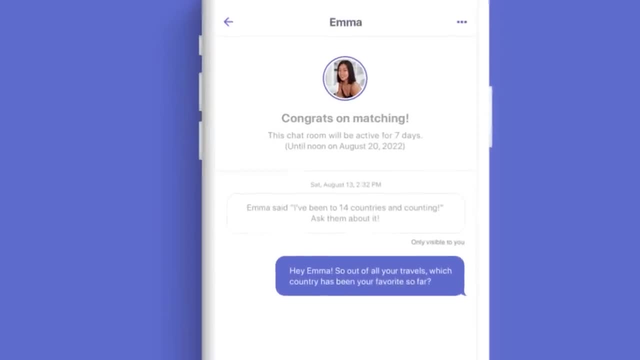 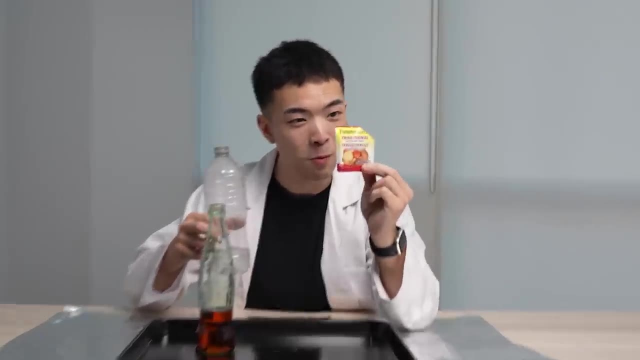 who work out and don't party. Also, they have an icebreaker feature, which makes it a little less awkward for you to slide in No more. hey, double whys. Now let's continue. We have our yeast, Let's add it to some warm water. 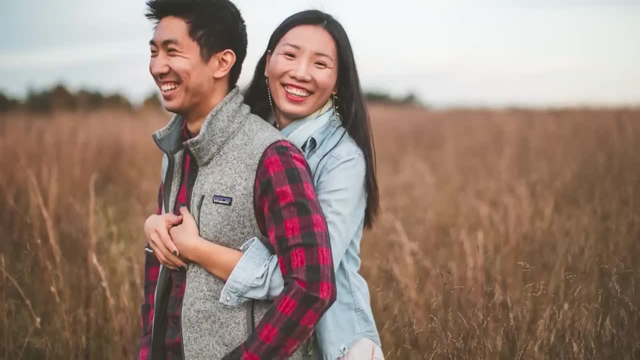 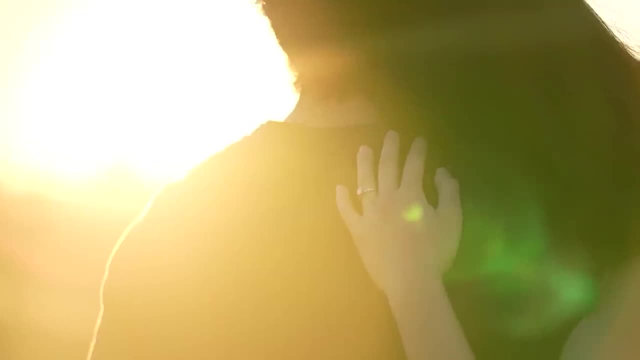 The yeast would be the catalyst that will start this chemical reaction. One of my friends from university actually found his girlfriend using Coffee Meets Bagel And from talking to all my friends that use the app, they vouch that the people on Coffee Meets Bagel 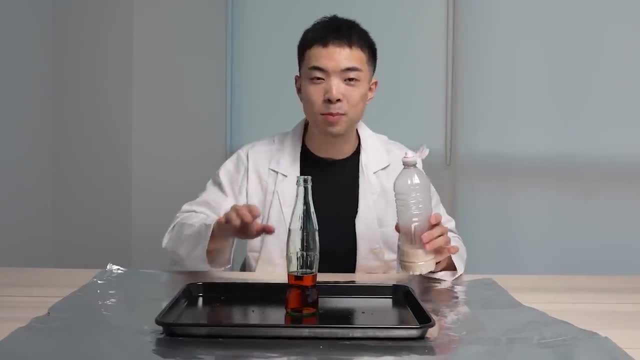 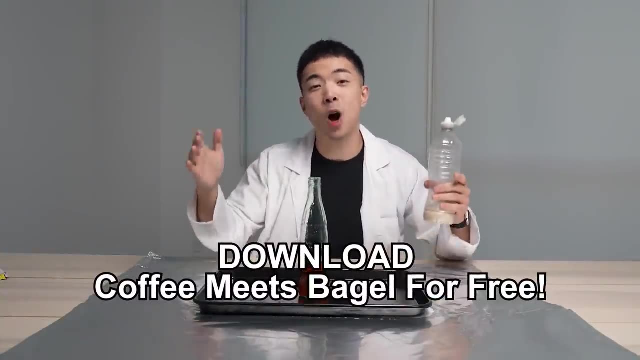 are a lot more wholesome than the other apps. Now this is the last step to our experiment. We add the catalyst into the solution that we made. If you're single and looking for a serious relationship, download Coffee Meets Bagel for free using the link in the description. 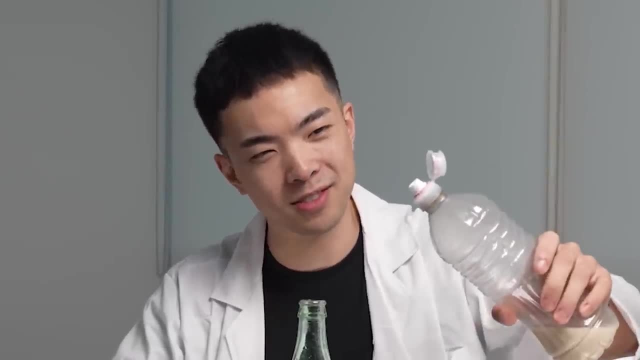 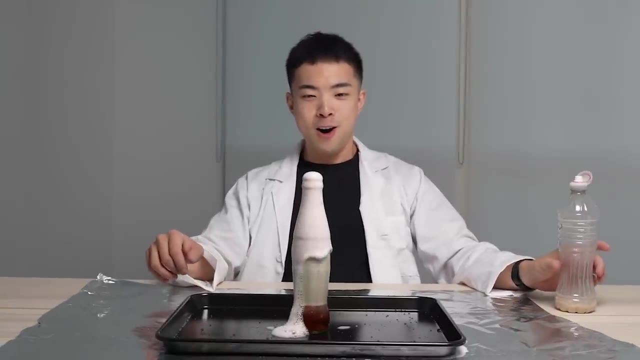 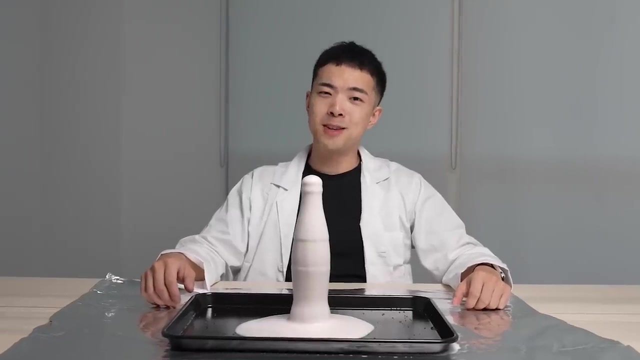 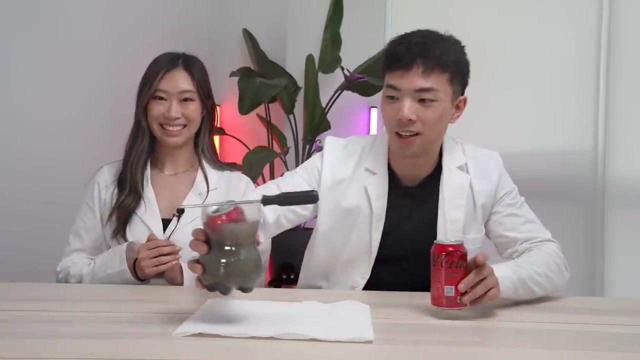 And get ready to start a chemical reaction of love. Whoa, Hopefully you don't explode this fast on your first date. All right, it's been over an hour. Let's check back on our aluminum can experiments Got the drain cleaner? one right here. 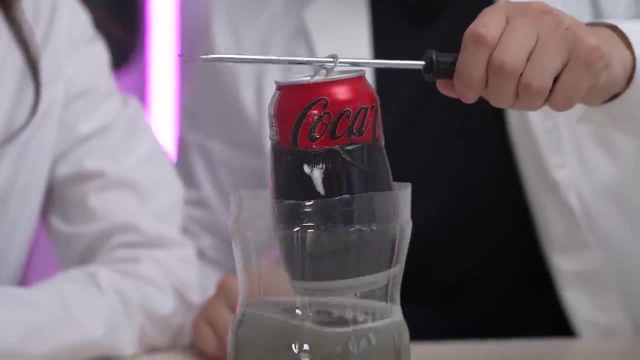 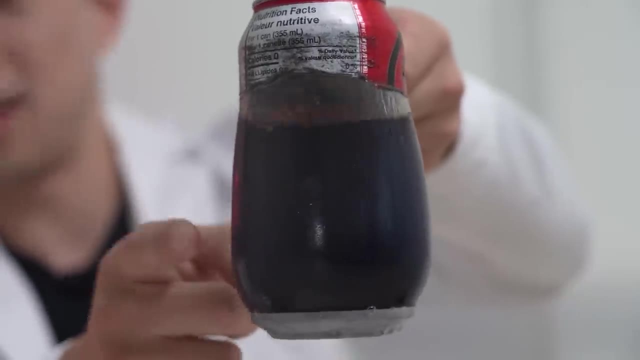 Let's pull this one first. Oh Good, Look at that, It's smokin'. So the drain cleaner has melted away all the aluminum And the only thing that's left is a plastic wrap inside. It's a sponging can. 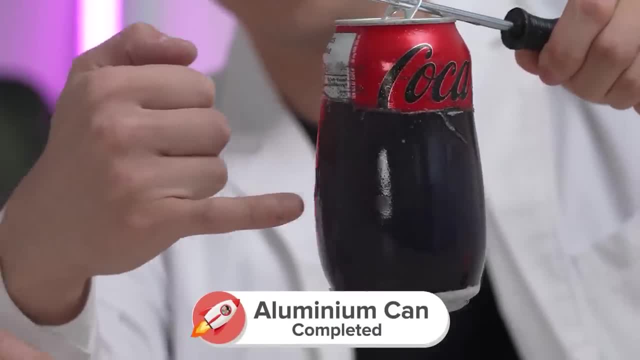 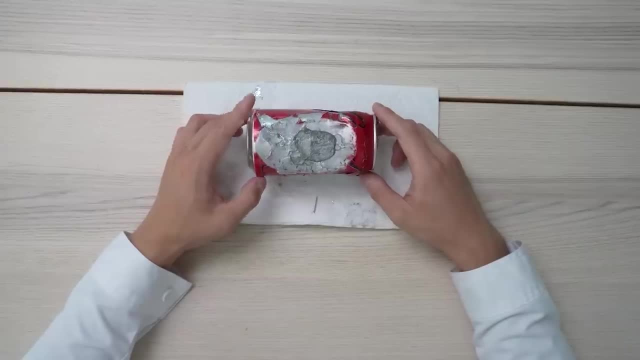 That's so cool. This is a gallium can. We left it there for a couple hours. I noticed some interesting textures. Let's see what happened. So, as you can see, this can has become destroyed. Let's just give it a little squish test. 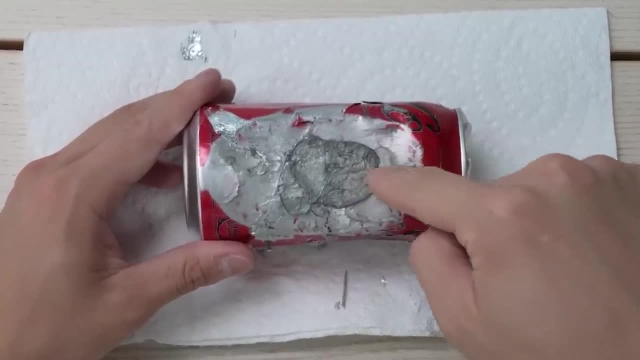 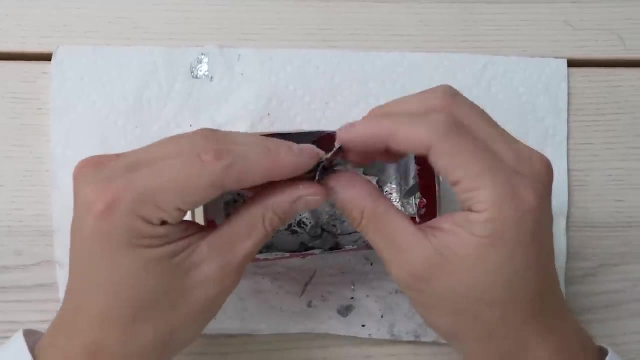 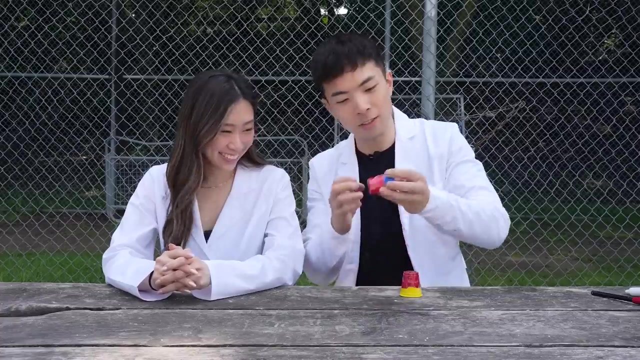 Wow, Let's try poking through with our fingers. Oh, Oh, my God, We can basically crumple this, can? It's like an aluminum croissant. Next, we have two tiny air guns, So how this works is literally just a cup. 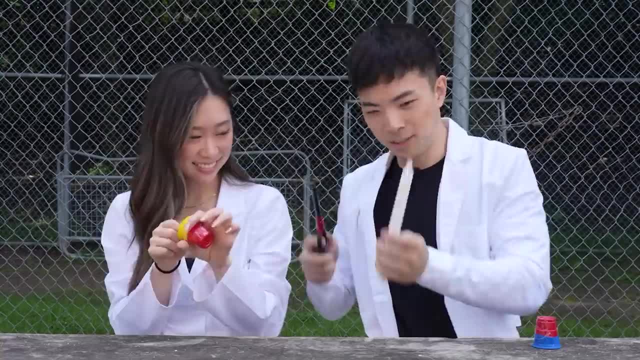 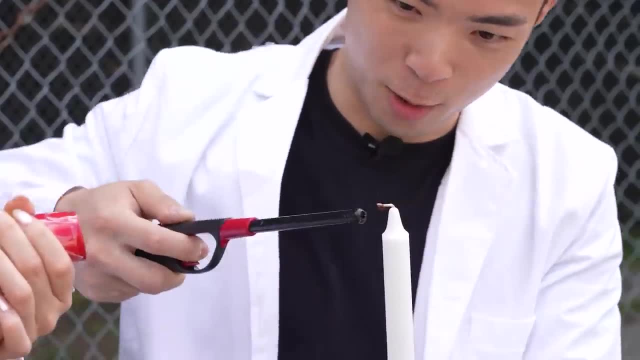 and a balloon attached to the back end. Do you feel that? Yeah, To see if it actually is working, let's light it on fire. Why does every experiment involve fire here? Cause fire is cool. Try blowing this up. There we go. 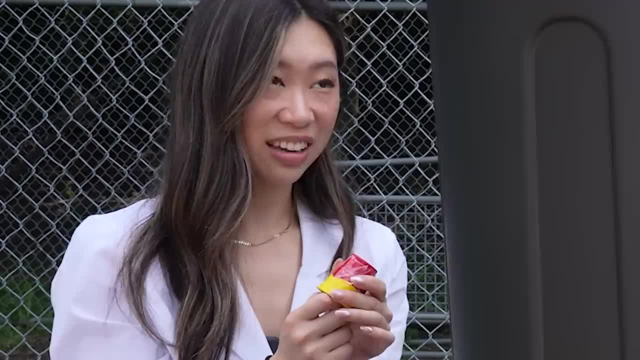 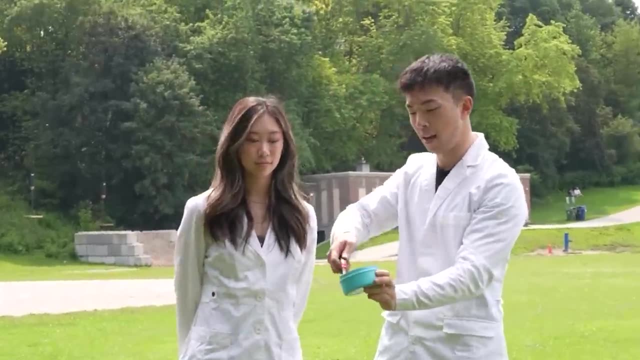 That was pretty cool, right? Yeah, Let's step it up a little bit. That's huge. What are we blowing with that, Your mom? So what we can do is actually we can just burn a little paper and it will become a smoke cannon. 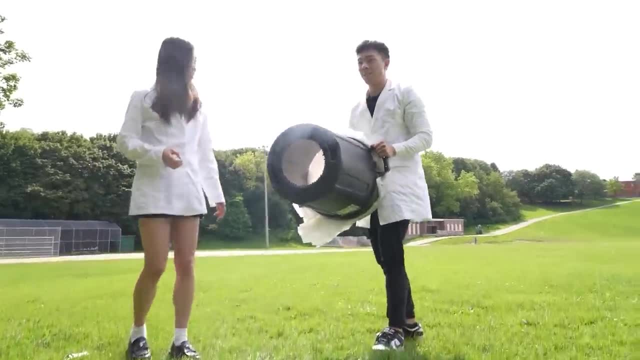 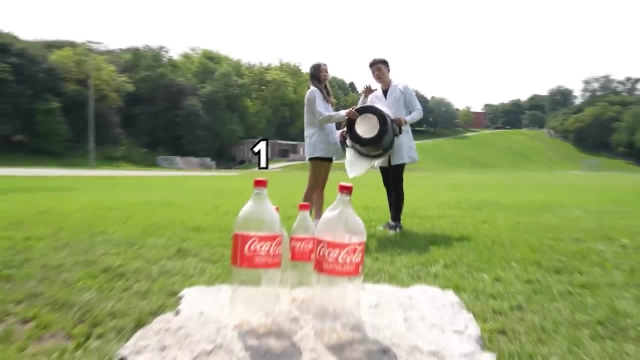 You can just put the paper inside. Our smoke cannon is now loaded with smoke. We can aim and fire it, So we got bottles set up over there. Here's the challenge: whoever knocks down the most number of bottles wins, and the loser has to drink lemon juice. 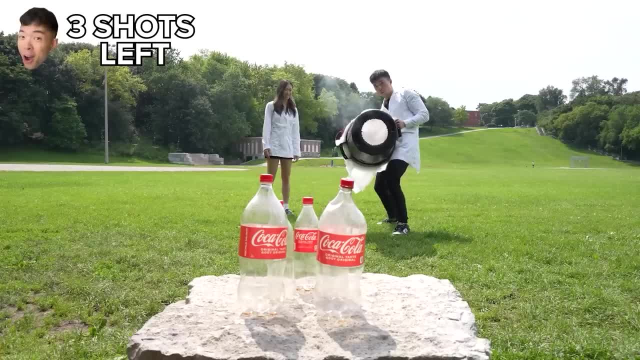 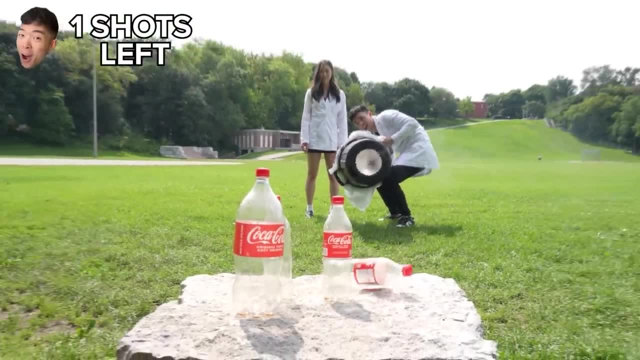 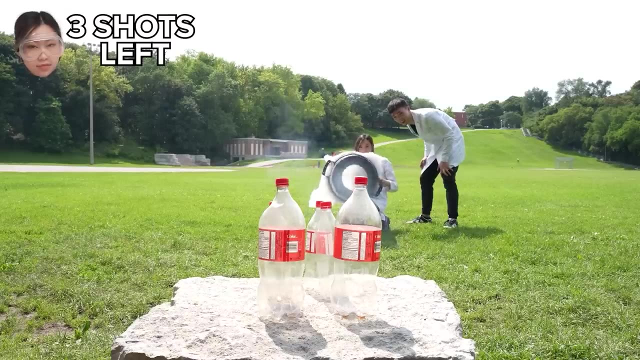 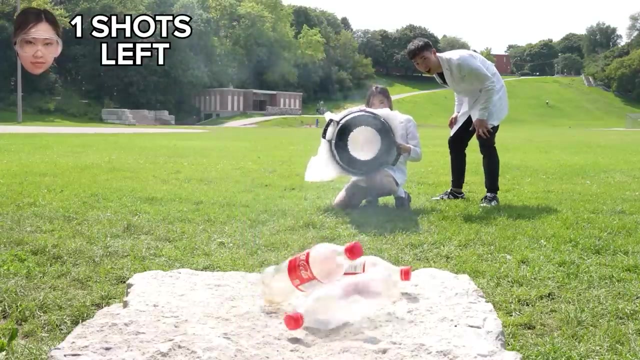 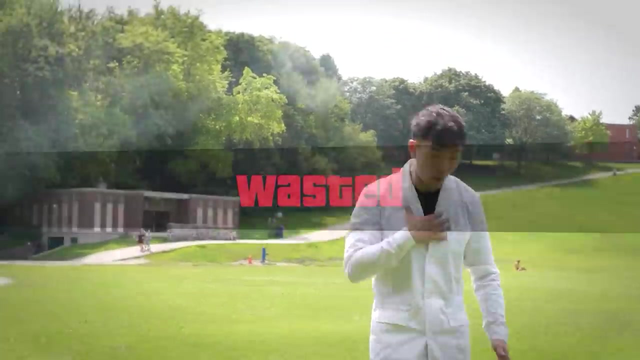 Okay, we get three shots each. Okay, Okay, I'll go first. Oh, You need to aim it a little lower. Okay, two down, Let's see if you can beat that. there we go, Shoot me, shoot me. I need to drink lemonade. This is lemon juice, It's not lemonade. 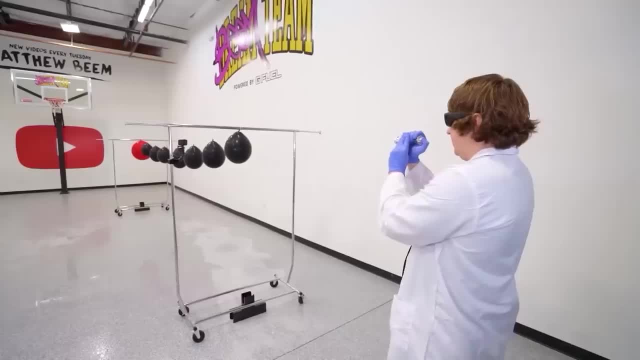 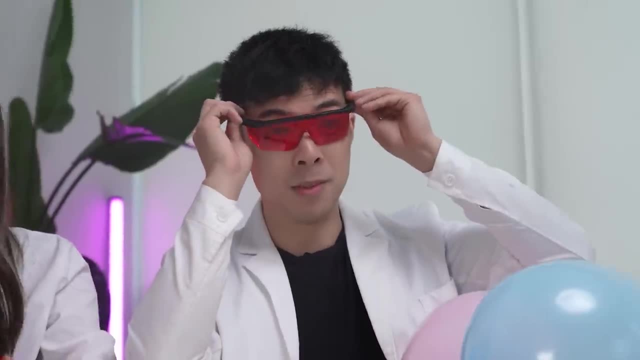 So sour, Holy crap. So this is the world's most powerful laser pointer. We need a different type of eye protection for this one. We need sunglasses. Mine are actually red because it cancels out the blue light from the laser. Let's test it on a balloon. 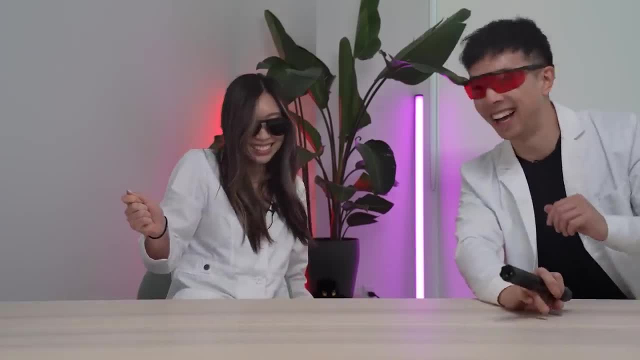 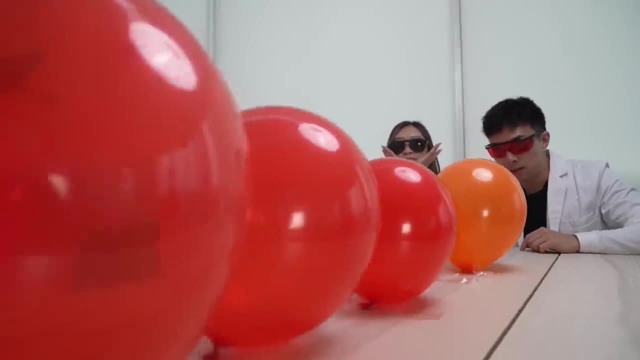 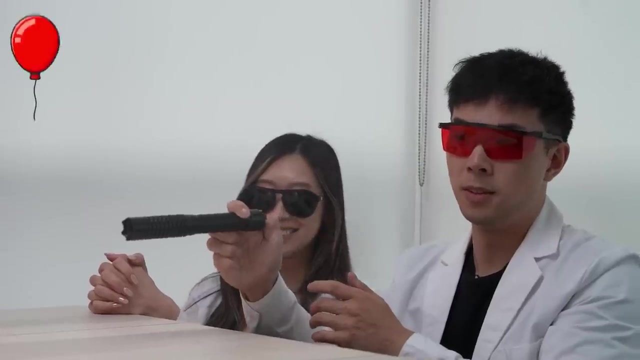 Oh, How many balloons do you think this laser will burn through? Three, I think it will burn through all these balloons. So I've even set up a match at the end to see if I can light that on fire. Okay, ready, Yeah, That's fast. three, four. 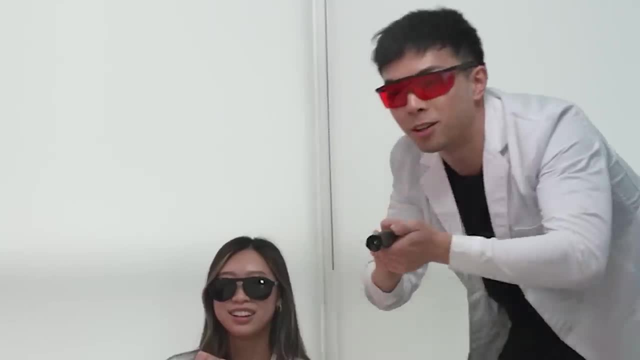 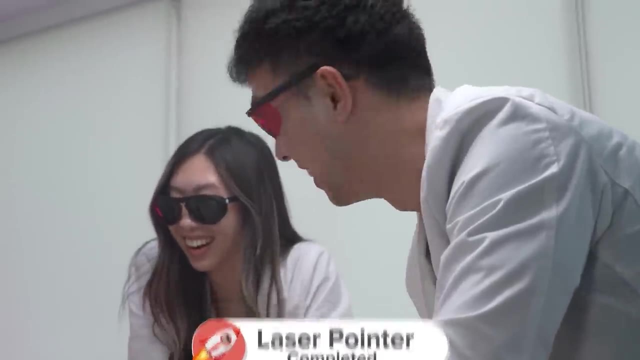 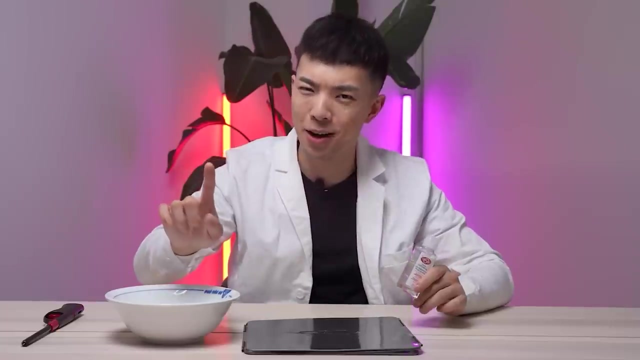 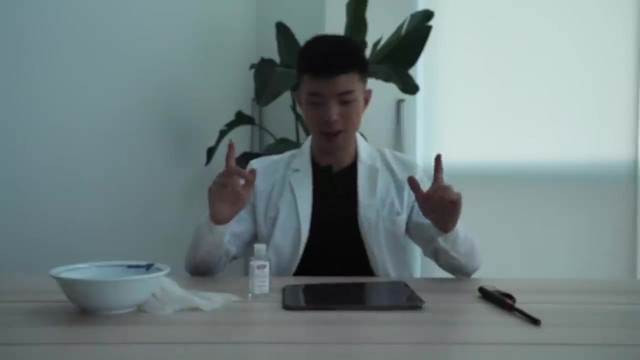 Six, seven, let me go a little closer. Cool, and it was only like 70 bucks Only. this next experiment only requires hand sanitizer. I'm sure you have some leftover, but don't try this at home. Extremely dangerous. It's called fire hands and in order for you to see this, we need to turn the lights off. 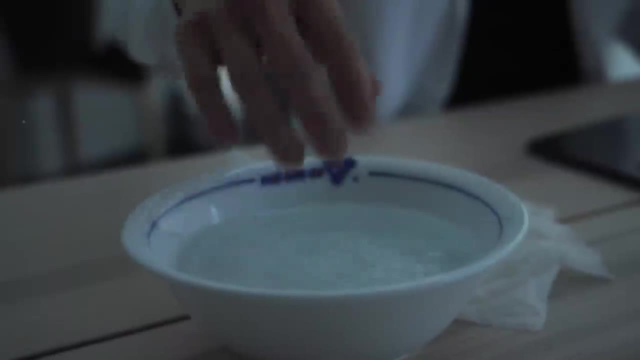 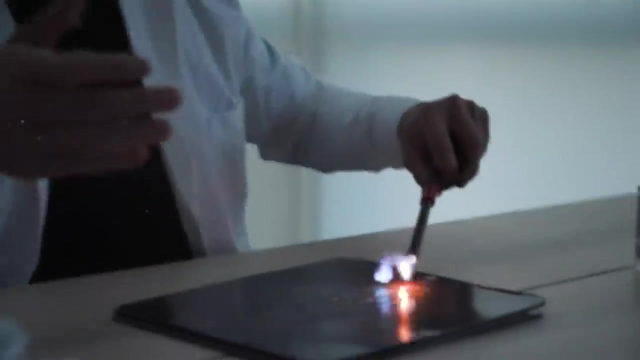 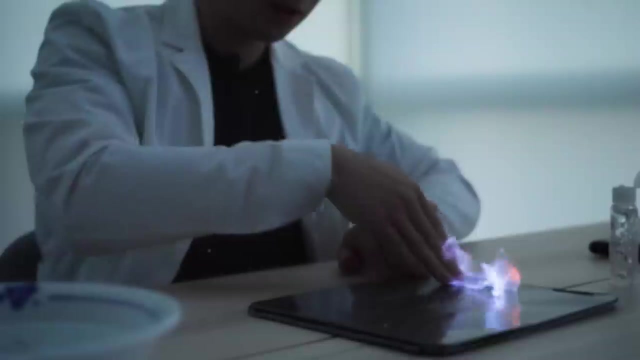 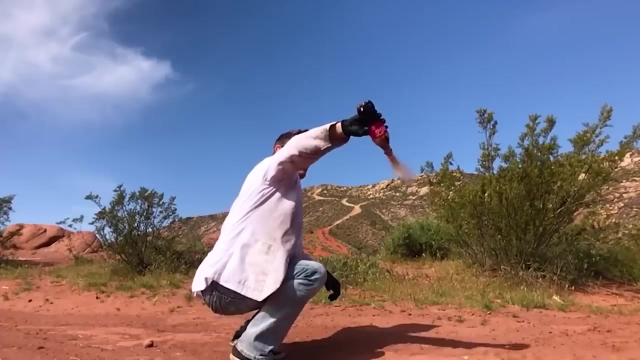 All right, that's better. first We're gonna squeeze the hand Sani onto our surface here, spread it around And then wet our hands so we don't burn ourselves. Hand sanitizer on a hand, Let's watch the magic happen. Onto the next experiment. 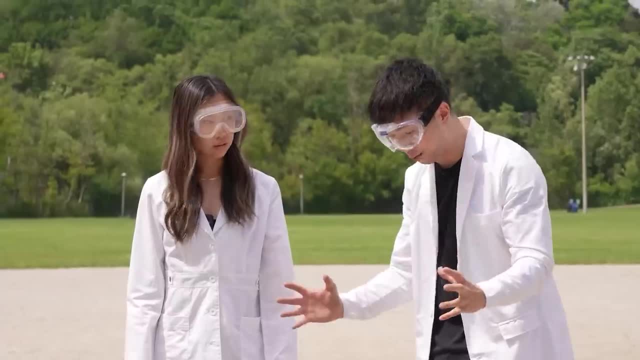 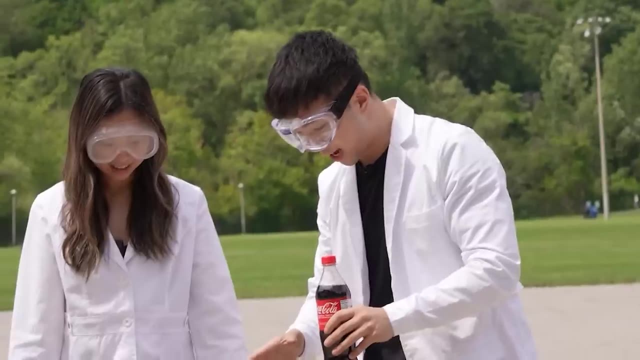 All right, now it's time for the final experiment. We're gonna use everything we've learned and combine it into a butane rocket. What does that even mean? A butane rocket? So butane when it's combined with Coke. 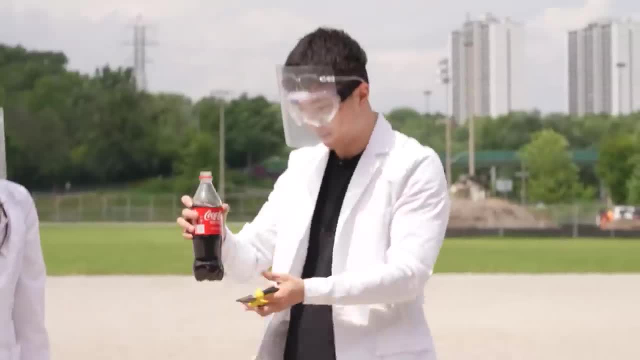 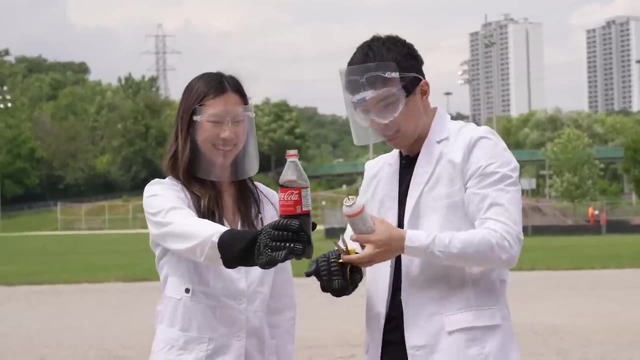 it will react at such a fast pace that it becomes rocket fuel. As my assistant, I need you to hold this. Yep, Wait, let me think about this. I don't wanna blow you up, Ah. So what I'm doing is I'm just letting the butane out. 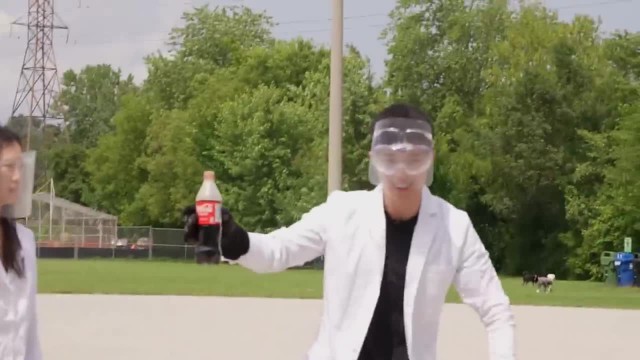 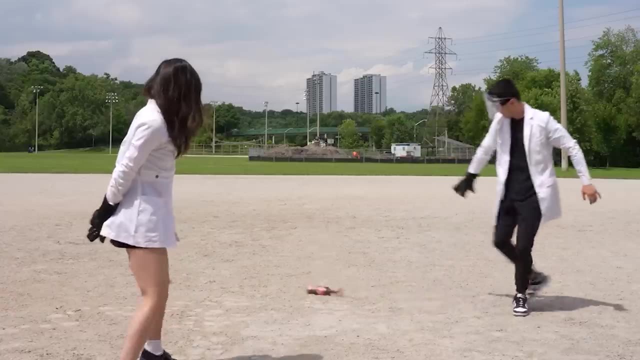 into the Coke bottle. We now have butane in this container. It is kind of smoking outside, as you can see. Can you see that? We're gonna see how this goes. One, two, three. Okay, we didn't have enough butane in there. 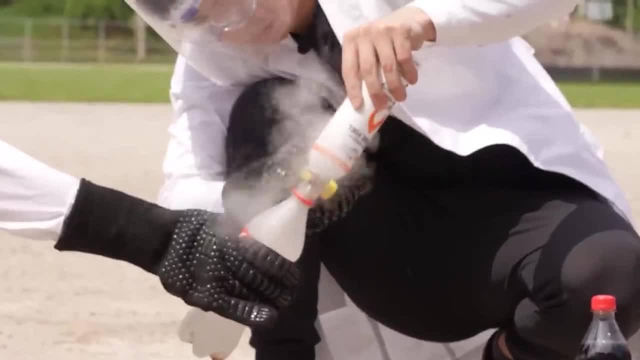 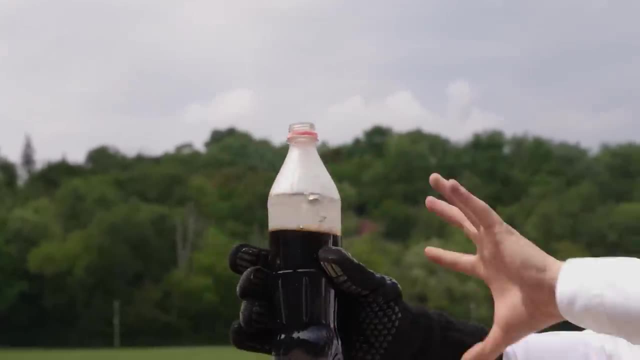 Okay. so what we're gonna do instead? we're first gonna fill up this Coke bottle with only butane and then we're gonna pour it into this Coke bottle. On top, we got a butane layer and then on the bottom, we got a Coke layer.